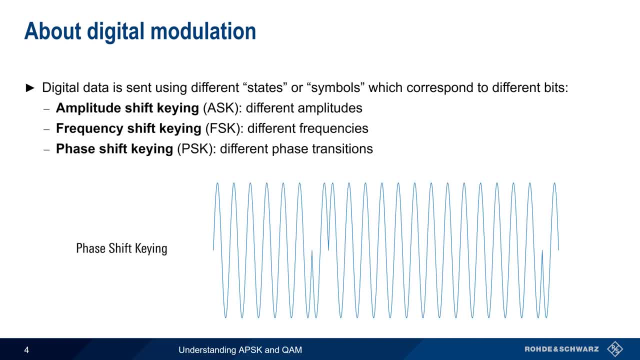 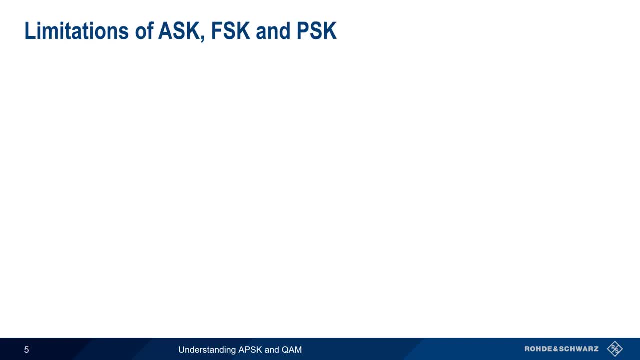 And in phase shift keying, sudden shifts in the phase of the received signal are used to indicate different states. ASK, FSK and PSK are widely used today, but mostly in applications that don't require high bit rates or throughput. These basic modulation schemes generally can't meet modern 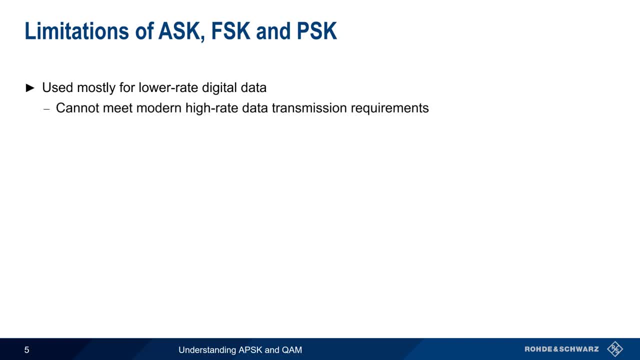 high data rate transmission requirements, such as those provided by Wi-Fi and cellular technologies. One way of increasing throughput is by increasing the modulation order, that is, the number of states or symbols. For example, we can increase the number of frequencies used in FSK to have more bits per symbol. In the case of two FSKs, we can increase the. 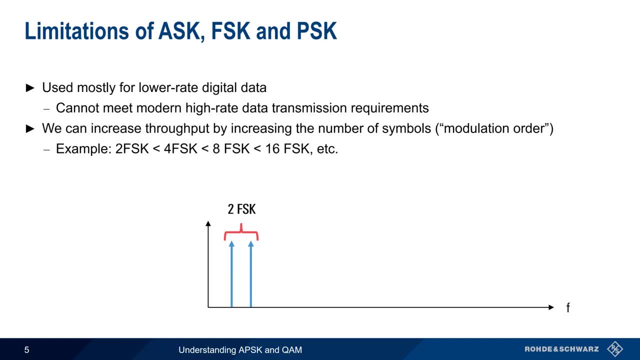 number of bits per symbol. In FSK or BPSK there's only 1 bit per symbol, 4 FSK has 2 bits per symbol, 8 FSK has 3 bits per symbol And 16 FSK has 4 bits per symbol, But there 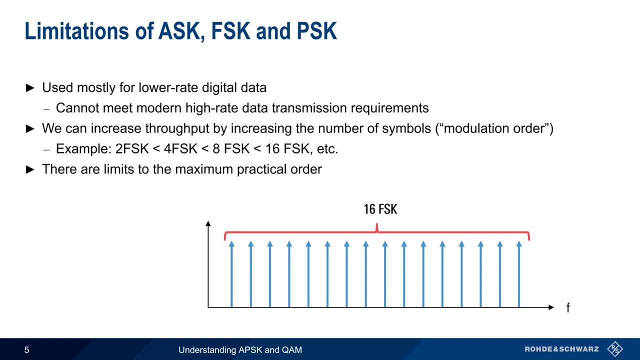 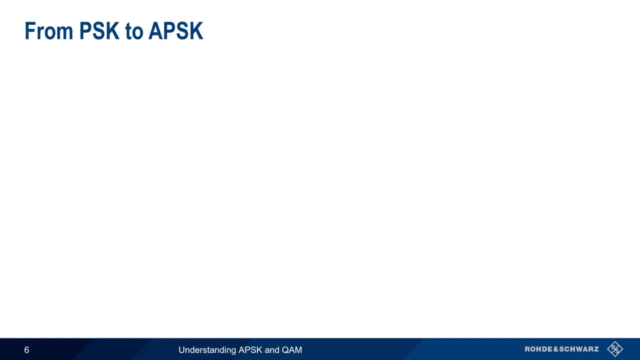 are some limits to the maximum practical order in these modulation schemes. ASK is very much limited by noise since it uses amplitude differences to represent different states And, as we can see, high modulation orders in FSK have wider bandwidth requirements. What about PSK? PSK also has a practical upper bound to modulation order Because 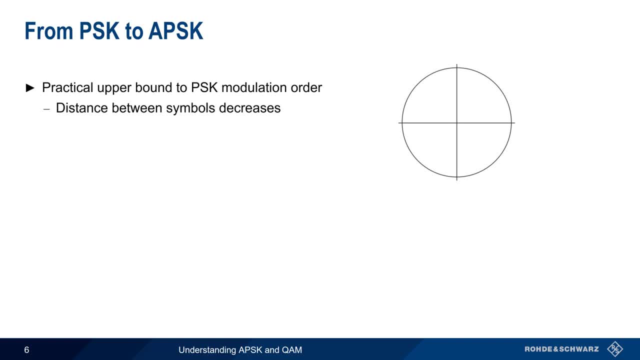 all the symbols lie on a single amplitude circle. the distance between the symbols decreases as the modulation order increases. When the states are very close together, errors become more likely. One solution to this problem is to add amplitude states. In other words, our constellation now has multiple concentric circles. each 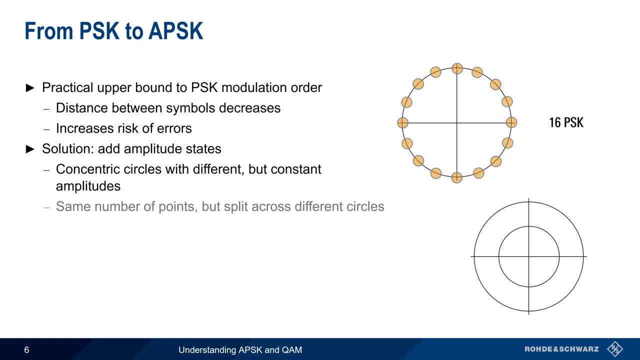 with a different but constant amplitude. We can then distribute the points across the field. We can then distribute the points across the field. We can then distribute the points across these different circles. so we have the same number of points, but they're further apart. 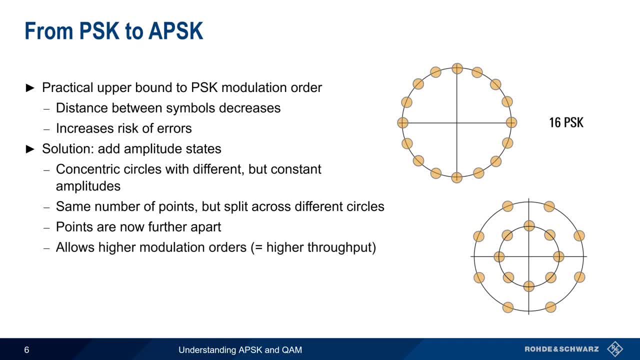 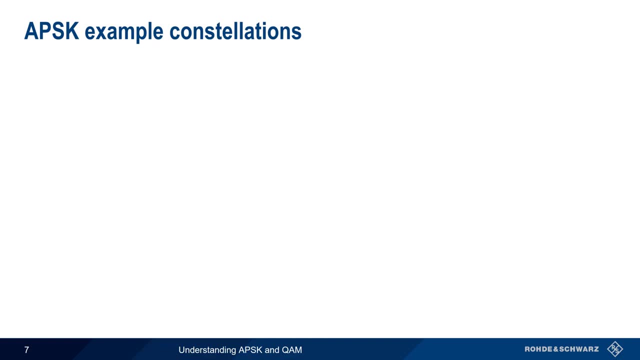 This reduces the risk of error and allows higher modulation orders, thus increasing throughput, Because we're now shifting between either amplitude and or phase descent symbols. this is called amplitude and phase shift keying, or APSK. Let's look at two example APSK constellations. In this 16 APSK constellation we have two. 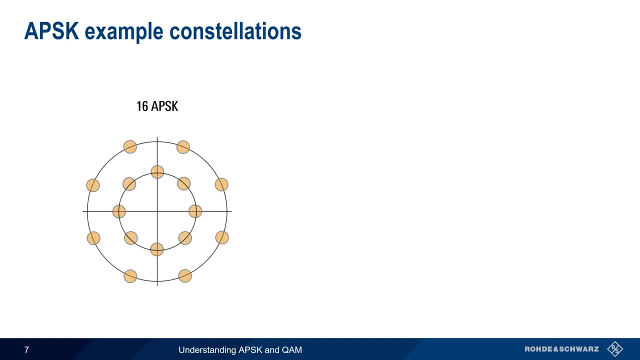 amplitude states and 8 symbols per state. 16 states means that each state can carry or represent four bits. This 32 APSK constellation has three amplitude states. The inner amplitude level has only 4 symbols. the middle amplitude state has 12 symbols and the remaining 16. 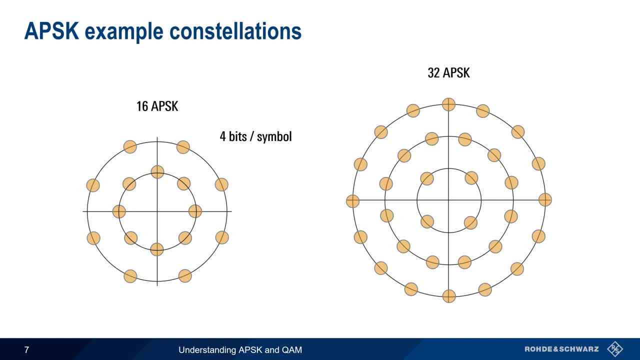 symbols are in the outer amplitude state. 32 states means that each of these symbols corresponds to 5 bits. Note, however, that other arrangements of the 32 symbols are also possible. Notice that the other arrangements of the 32 symbols are also possible. 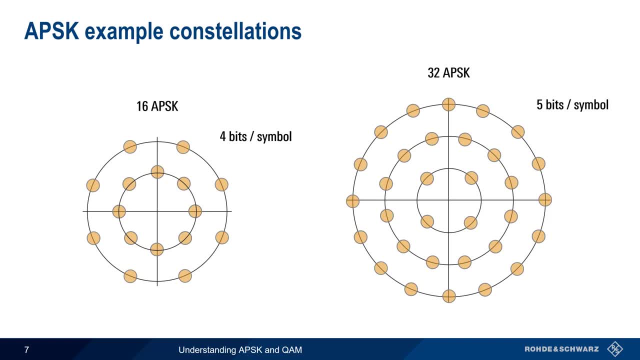 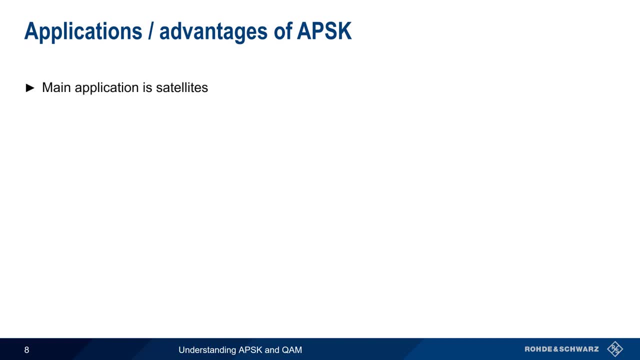 Note that the other arrangements of the 32 symbols are also possible, such as a 32 APSK constellation with four amplitude levels. Satellites are probably the most important application of APSK, and APSK is part of the DVB-S, or digital video broadcast. 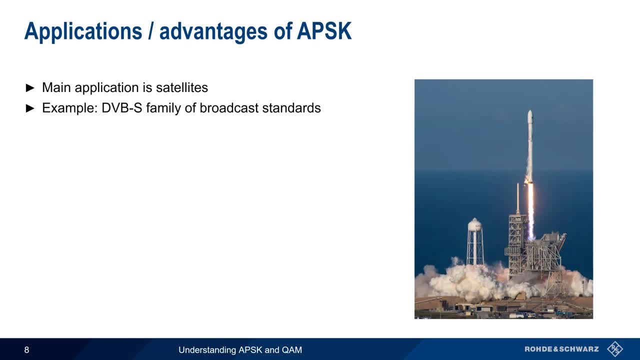 satellite specifications. In addition to other modulation types, the DVB-S2 standard includes support for 16 APSK and 32 APSK. The newer DVB-S2X standard adds support for 64,, 128, and 256 APSK. 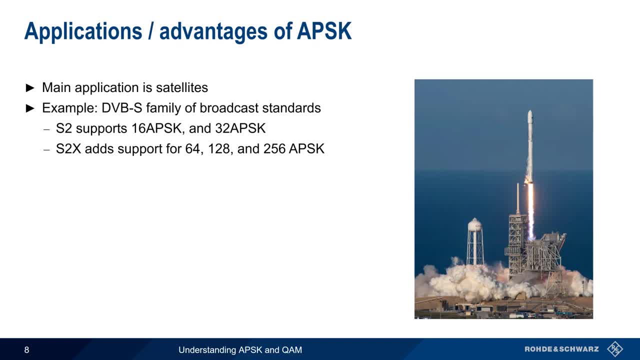 One of the main reasons for using APSK in satellite applications is that APSK is robust with regards to various amplitude effects and it allows the use of non-linear amplifiers. For example, non-linearity, such as compression, may change the relative distances between different 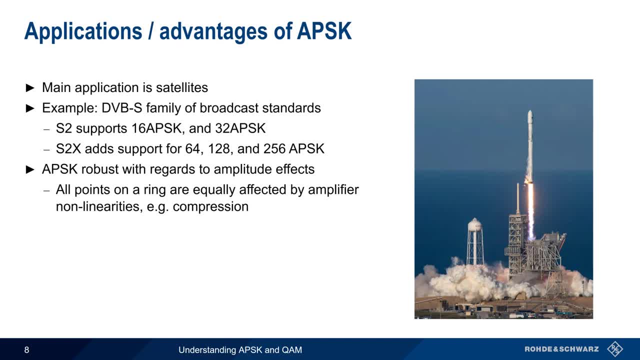 amplitude rings, But all the points in one given amplitude ring will be equally affected, which minimizes the impact of this non-linearity. In fact, APSK allows the distances between the rings to be pre-distorted so that the rings are the correct distance apart after non-linear 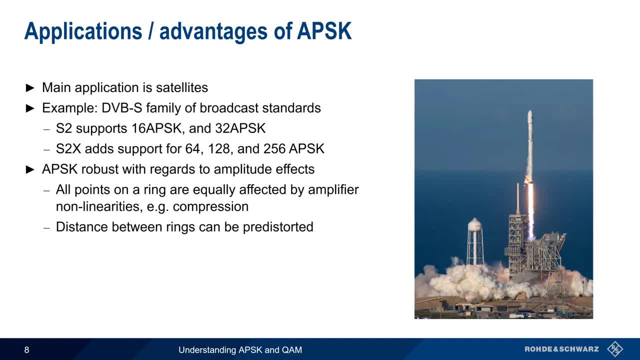 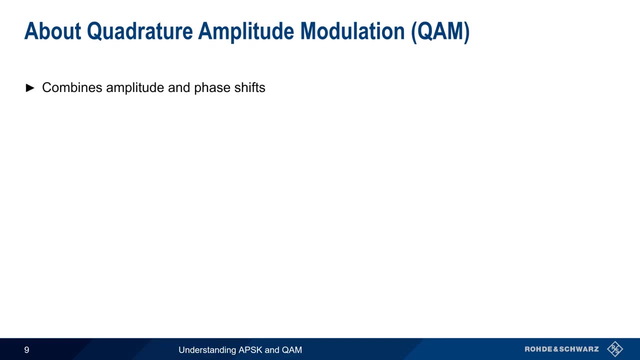 amplification. APSK provides further flexibility, in that the number of rings and the distance between the rings can also be chosen or adjusted in order to balance distortion versus peak-to-average power ratio. Another form of modulation that combines amplitude and phase shifts is something called 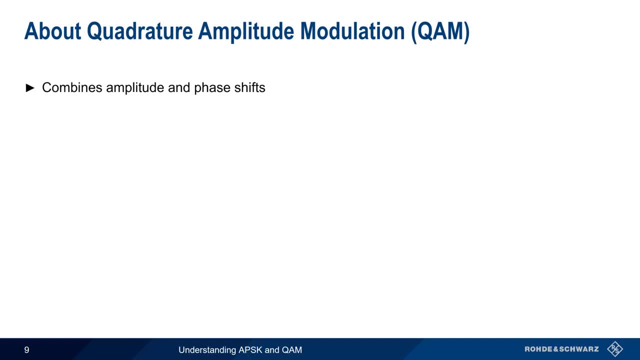 quadrature amplitude modulation or QAM. Many digitally modulated signals – especially higher order signals – are created using something called I-Q modulation. An I-Q modulation in-phase or I-component is combined with a quadrature or Q-component to produce a modulated signal. Quadrature simply means shifted by 90 degrees. 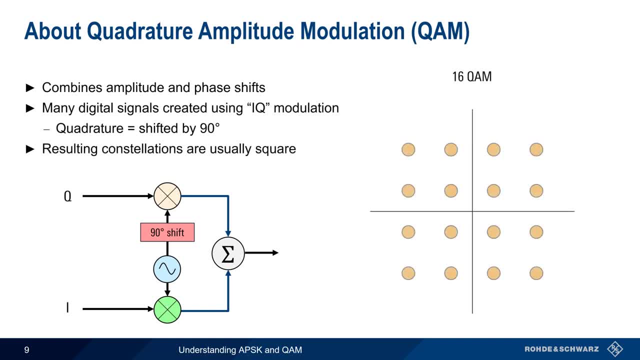 The result of this I-Q modulation is a constellation diagram, But the points are arranged in a square shape, each point having a unique combination of amplitude and phase. In this example, our 16 QAM signal carries 4 bits per symbol. If we increase the modulation order or number of states to 64, each point in the resulting 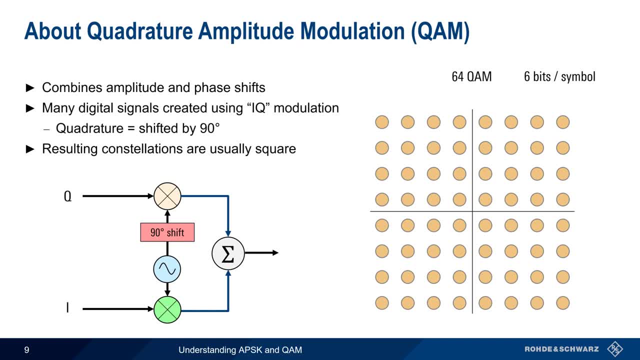 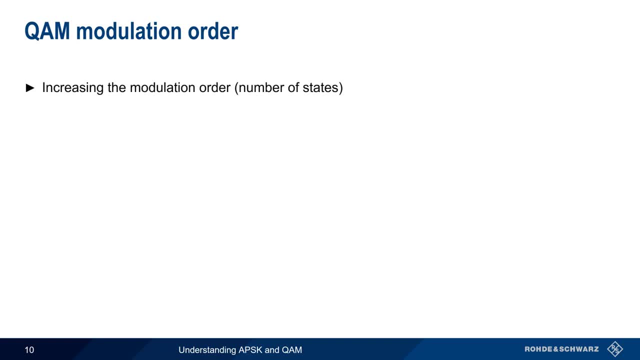 64 QAM constellation now corresponds to 6 bits. Recall that increasing the modulation order or number of states has two main effects. First, the higher number of bits per symbol mean that the achievable bit rate, or throughput, also increases. 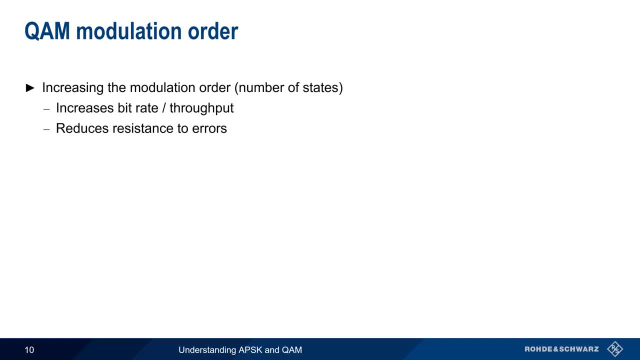 On the other hand, higher order modulation also reduces resistance to errors, since the states or symbols are now closer together. That said, QAM is capable of supporting very high modulation orders. Some of the more common QAM variants are 16 QAM, 64 QAM, 256 QAM, 1024 QAM and 4096 QAM. 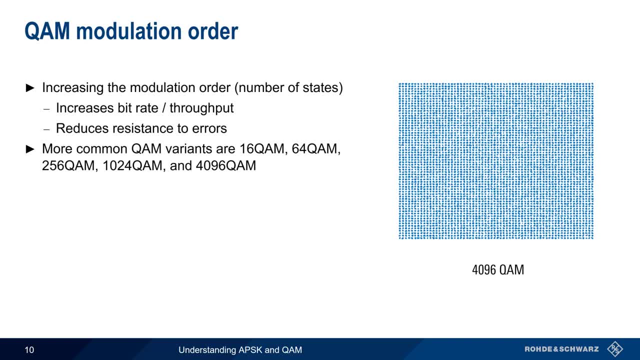 although other orders are possible, Using 4096 QAM as an example, this very high order modulation scheme represents 12 bits with every symbol, so the data rate is quite high. However, we can also see that the constellation points are very close together, so the probability 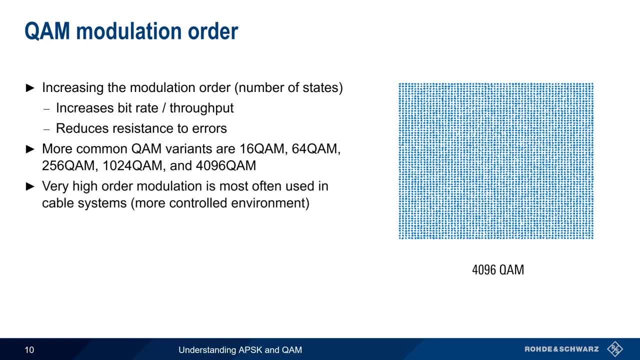 of error is also much higher. Therefore, very high order QAM modulation tends to be used most often in cable systems, where the environment is more controlled and less susceptible to noise and interference Over the air. applications such as sub-satellites and other environments. QAM modulation is 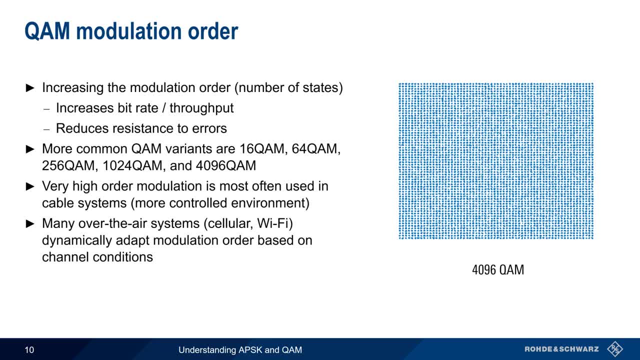 more controlled and less susceptible to noise and interference. Local and interlaced satellite systems, for example, often dynamically adapt modulation order based on the channel conditions, For example using 256 QAM when conditions are good, but falling back to 64 QAM or 16. 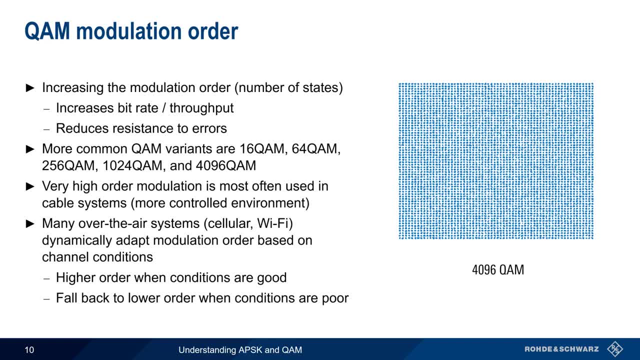 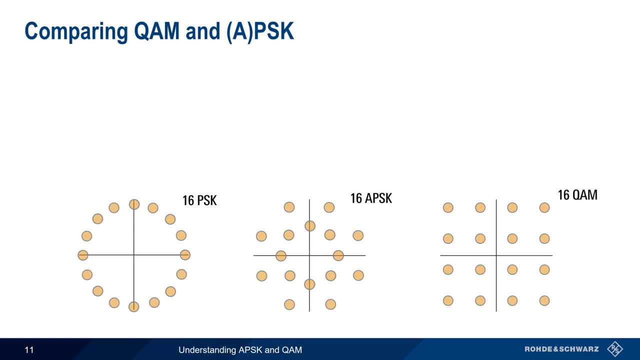 QAM in the presence of noise interference, etc. So let's compare PSK, APSK and QAM, all using the same modulation order. All three of these constellations have 16 states and all of them transmit 4 bits per. 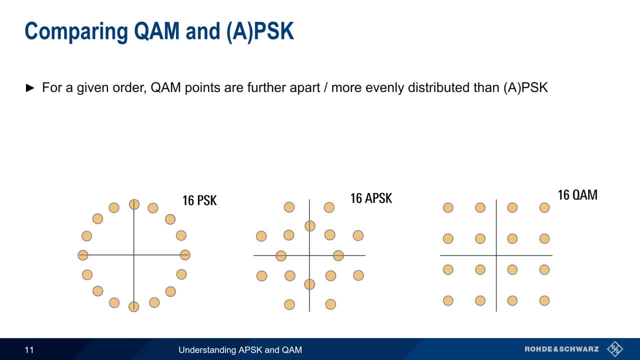 symbol. Note, however, that the QAM points or symbols are spaced further apart and are more evenly distributed than both PSK or APSK. As we've mentioned a few times already, more distance between the points means more resistance to error. Another important difference is the number of amplitude states. 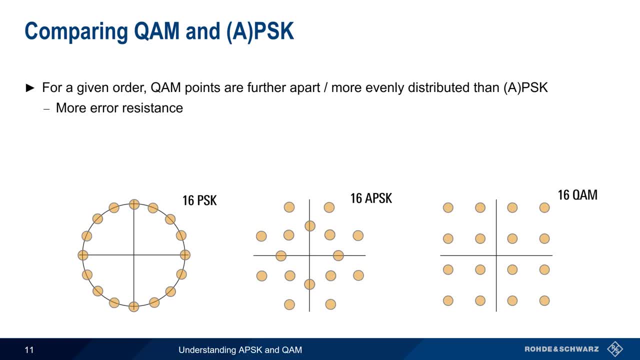 16 PSK has only a single amplitude state, 16 APSK has two amplitude states and 16 QAM has three amplitude states. Recall that increasing the number of amplitude states places higher linearity requirements on amplifiers and transmitters due to higher peak-to-average power ratios. 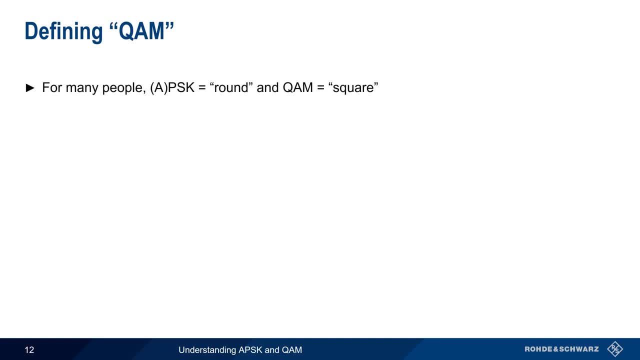 For many people, the difference between QAM and APSK is that APSK constellations are round and QAM constellations are square. However, the term QAM is also used generically to refer to any modulation that defines symbols using IQ modulation. 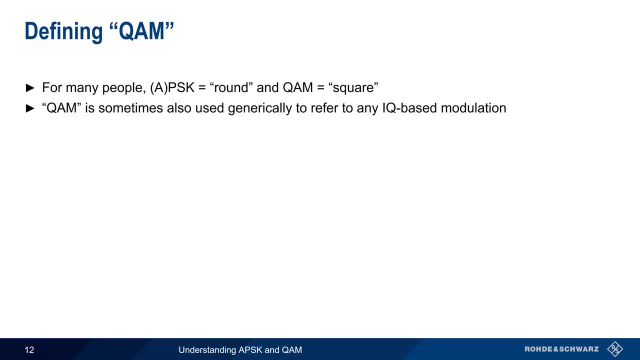 and not all of the resulting constellations are the same. However, the term QAM is also used generically to refer to any modulation that defines symbols using IQ modulation, and not all of the resulting constellations are the same. For example, the wideband HF specifications refer to this constellation as 16 QAM. 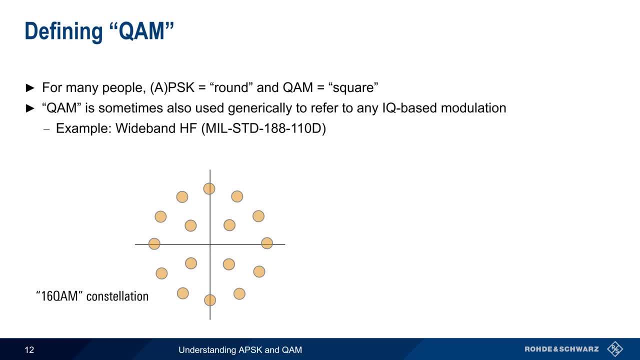 for example, the wideband HF specifications refer to this constellation as 16 QAM, although it actually consists of two PSK rings- an inner 4 PSK ring and an outer 12 PSK ring- although it actually consists of two PSK rings- an inner 4 PSK ring and an outer 12 PSK ring. 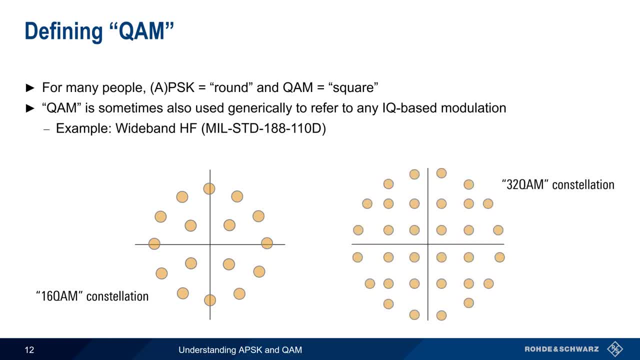 Likewise, this 32 QAM constellation from the same specification consists of an outer ring of 16 symbols ranged in a PSK-like circle and an inner square of 16 QAM-like symbols, But in most cases the PSK round- QAM square distinction is a reasonably good rule of thumb. 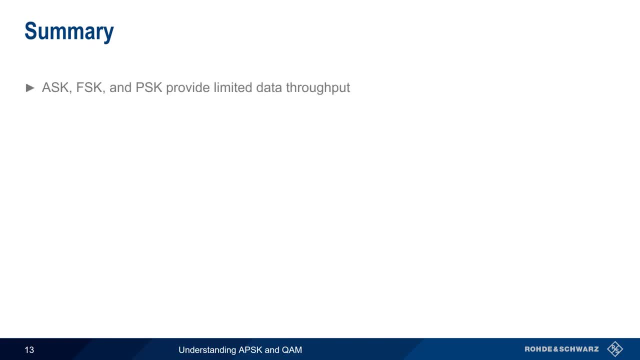 Let's summarize what we've covered. Basic digital modulation schemes like ASK, FSK and PSK are still widely used for low data rate applications, But by combining both amplitude and phase modulation much higher throughput can be achieved. In APSK, additional amplitude states are used to space the symbols further apart, allowing 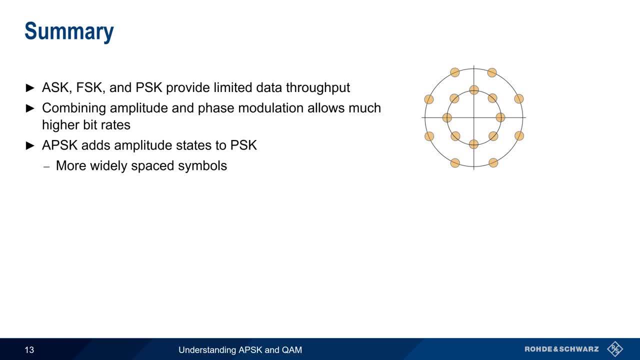 for higher modulation orders and acceptable error rates. APSK still maintains a relatively low peak-to-average ratio, making it a good choice for satellite applications such as DVBS. Another form of amplitude and phase modulation is QAM, which is based on so-called IQ modulation. 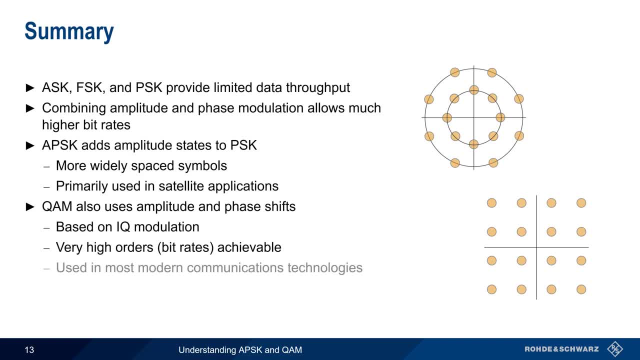 Very high modulation orders are possible with QAM, meaning that QAM is the modulation scheme of choice for most terrestrial data communications. This concludes our presentation Understanding APSK and QAM. If you'd like to learn more about test and measurement solutions for digital modulation,